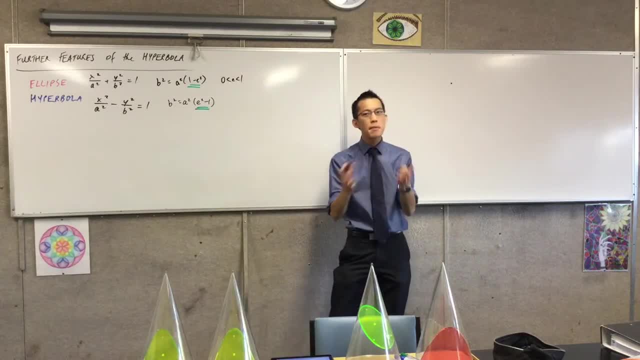 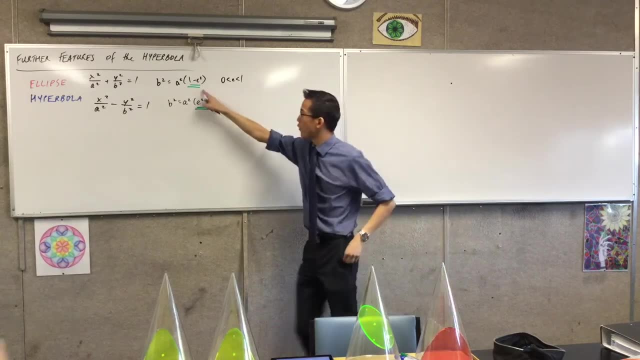 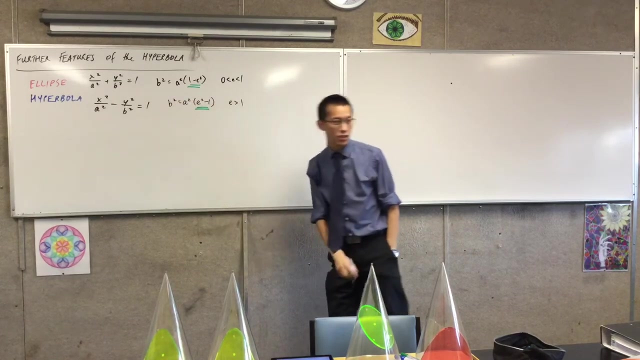 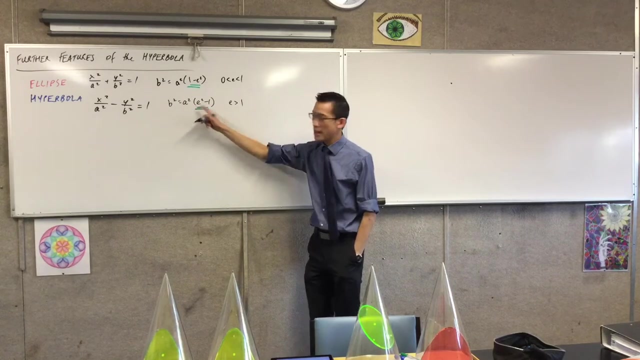 0 to 1, right, then it must make sense that e is going to be a small number, like it's a fraction. you square it, it gets smaller, and so in order for everything to stay positive here, you've got to have 1 minus e squared. whereas if e is going to be some big number, like 2 or 3 or 500, then in order for things to stay positive- mainly for b to stay positive, b squared, then e squared has to be up the front, okay. 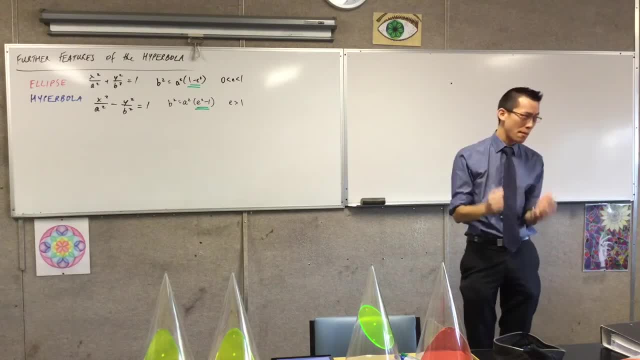 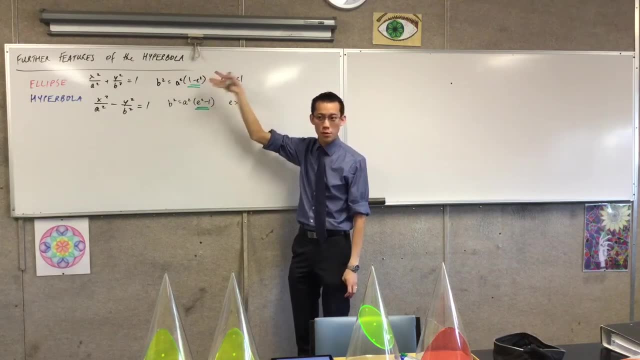 Please get that there's meaning behind this order. Please do not memorize these as meaningless algebraic statements. okay, Now, once you've used these like, let's go back to ellipses, which we're a little more familiar with. we spent a good deal of time on them. 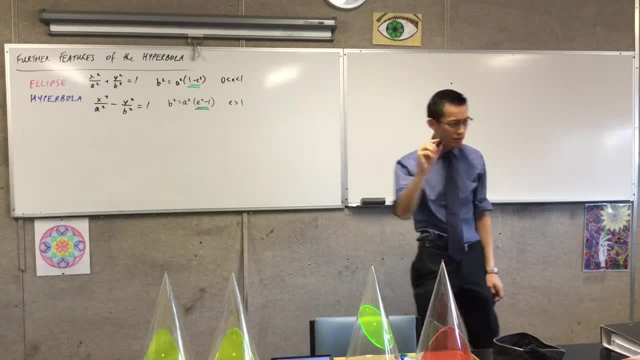 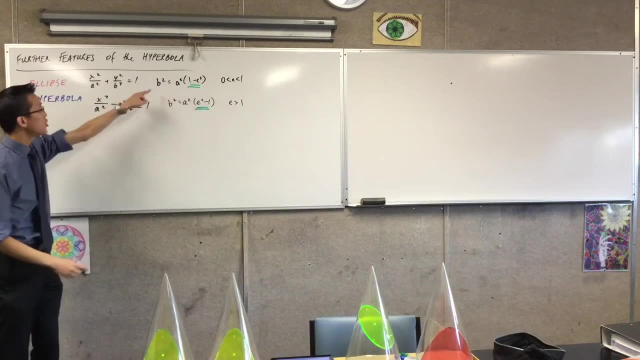 What do you then go ahead and do once you start with that line? What do I do after that? Okay, yeah, very good, I'm going to go from here, right, I'm going to punch in whatever a and b might be- 9,, 16,, etc. 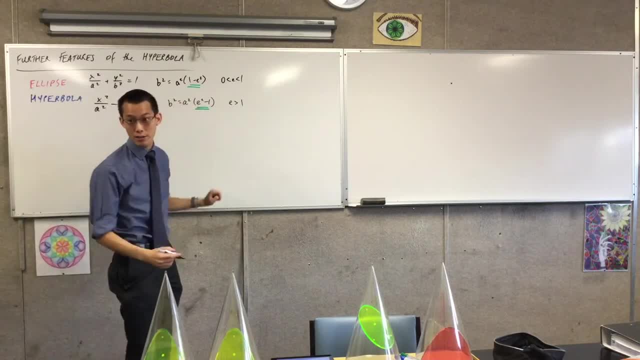 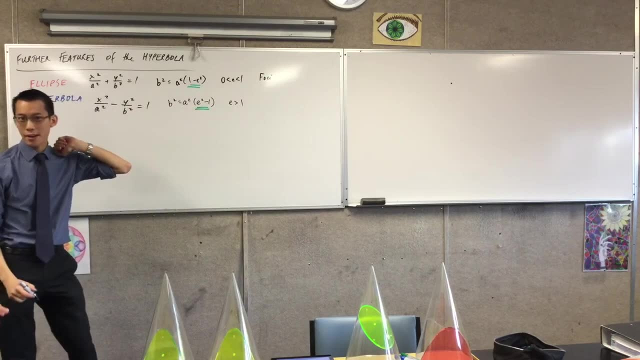 And that'll give me the eccentricity which I then use to find the furcane directrices. These are the main features, right? So this is the photoki we can find at. this is in the ellipse they're at. where are they? 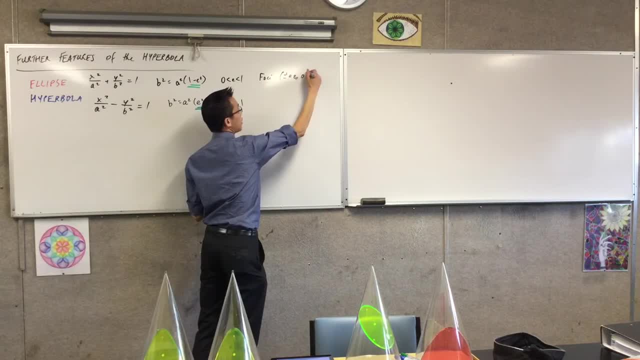 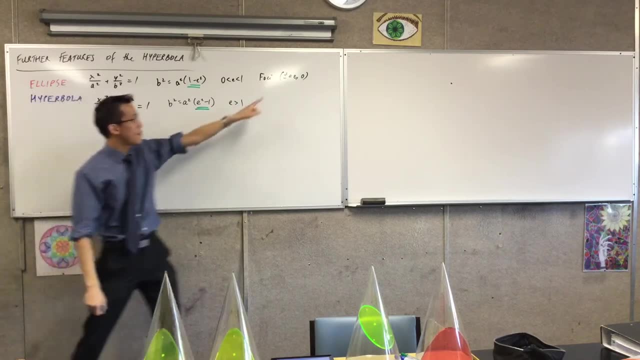 Plus or minus a e comma 0, and of course this is- we're all thinking just in standards at the moment, like the original ones. so this is horizontally oriented right. So that's why my photoki have gone that way and the directrices are where. 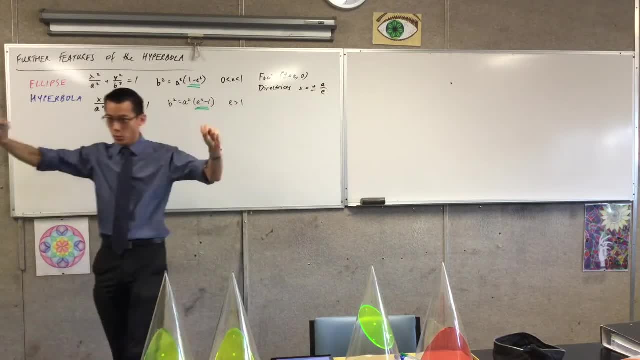 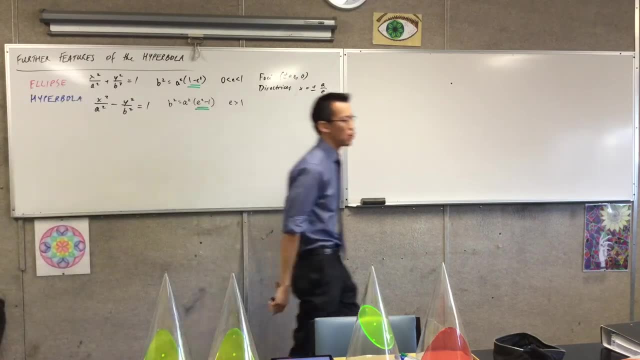 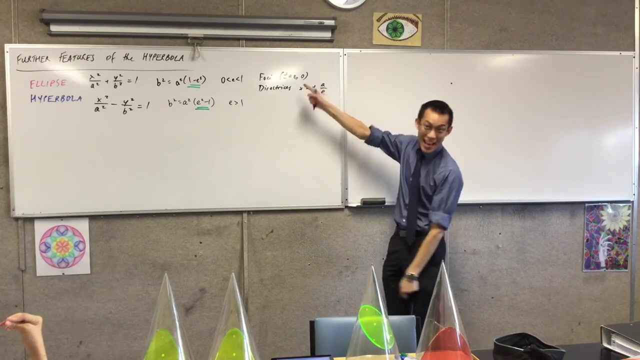 Very good. So again, they've gone this way and I've got these vertical lines happening on the outsides of my ellipse. okay, Now, mercifully- and I didn't bother going into the geometry of it, because it ends up being number one, quite repetitive number two- you never need to know the proof number three: you end up with the exact same answer. 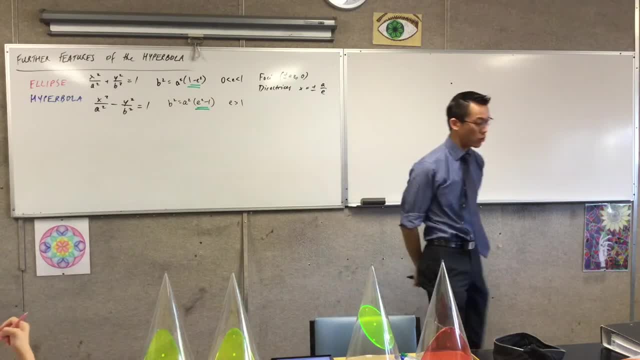 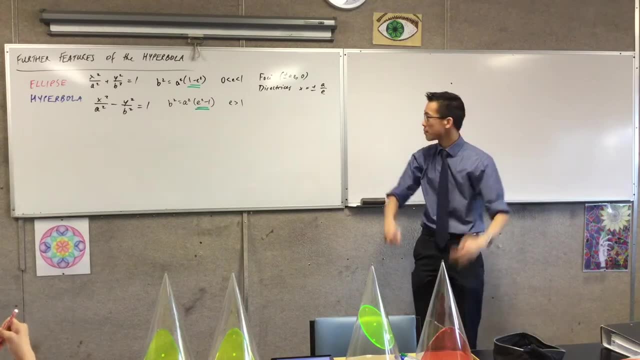 The furcane directrices for the hyperbola. are those coordinates? okay, But the hyperbola has more features than the ellipse because of the geometry of its shape. For instance, we noticed that there were acetones, Acetones. 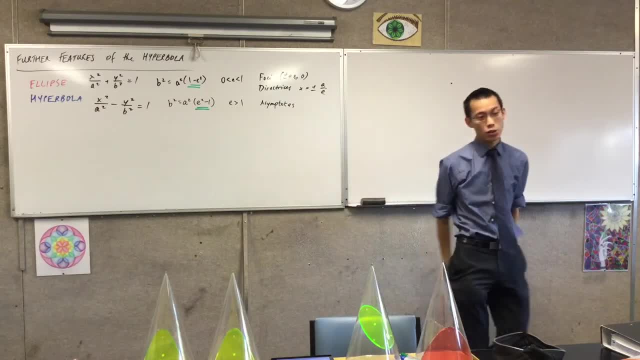 And whenever you grab something with acetone, you notice that there's acetone. When you find acetones, it's important that you state what the acetones are and you show them then, okay, I'm going to show in a minute how you find what the acetones are. 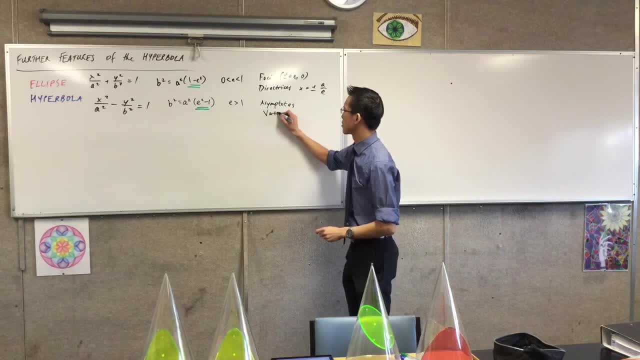 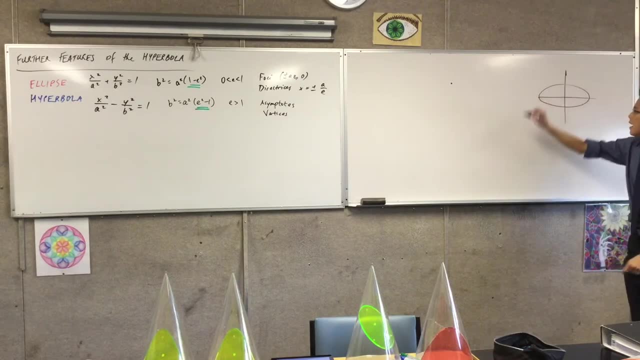 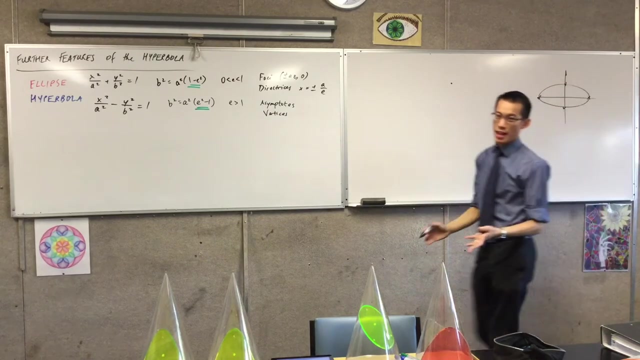 There's one other feature that's important, and they're called the vertices. right Now, for an ellipse, you would say I've got a shape and it intersects with the coordinate axis, So I've got one, two, three, four intercepts for a regular ellipse that's centered on the origin. 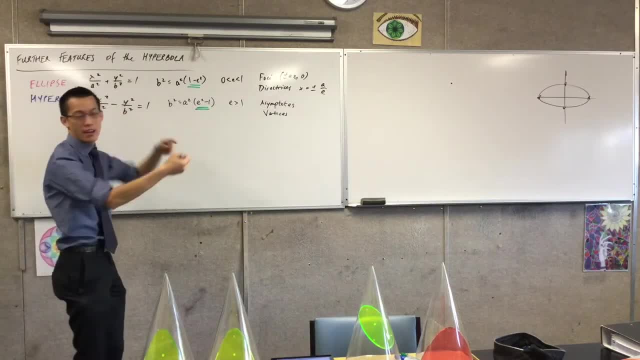 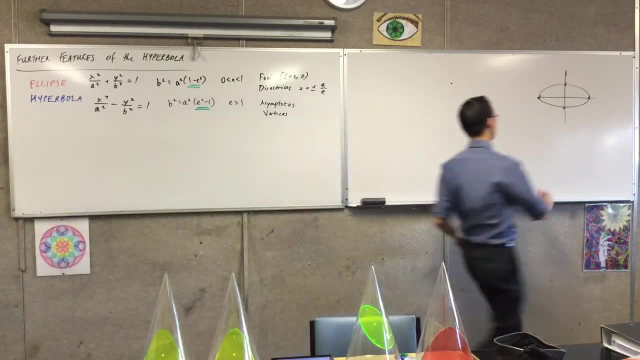 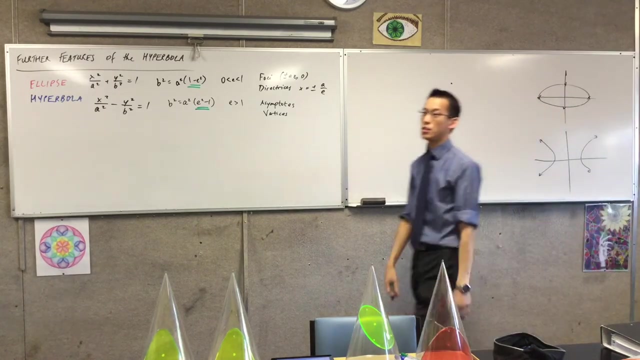 Obviously, if it's not centered on the origin. if I move somewhere it might have no actual intercepts, but those are still the critical points. But for a hyperbola the intercepts are not just intercepts. They represent a change in the behavior of a hyperbola right. 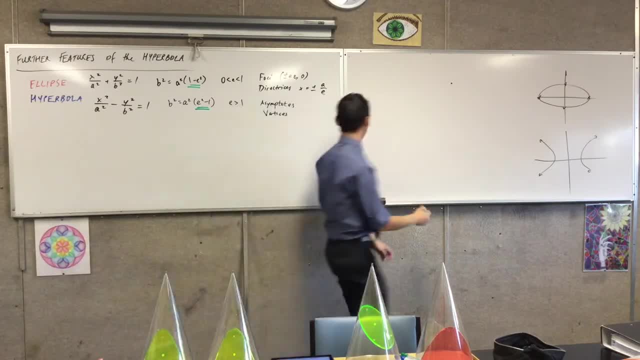 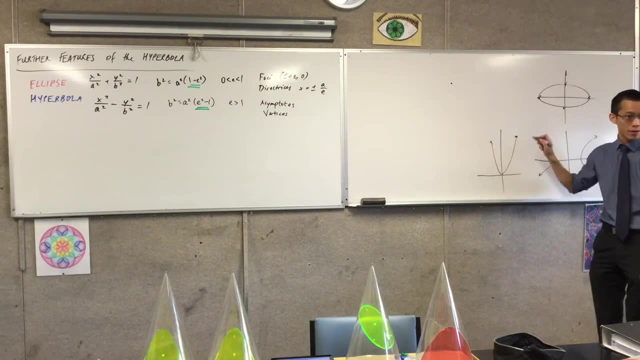 In fact, it's the same behavior that we see in a parabola right. Where's that? It's a turning point? okay, Now, being that these are- and I'll put it in inverted commas- these turning points are oriented horizontally right. 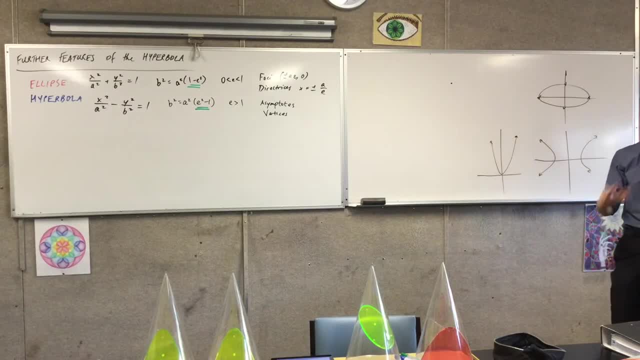 You can't really call these turning points the way we would think about them in calculus. okay, Because there's not a change from like negative gradient to positive gradient. There's not even a gradient in here, And the gradient is two different things here because it's a relation, right? 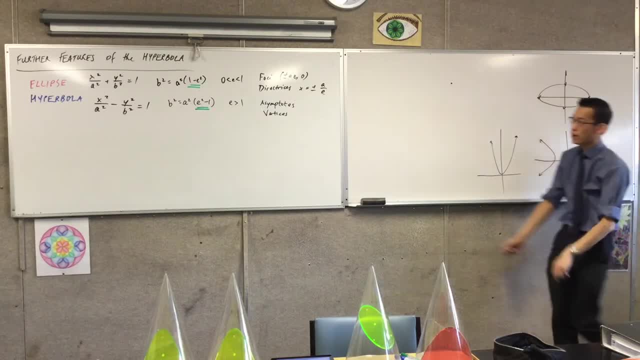 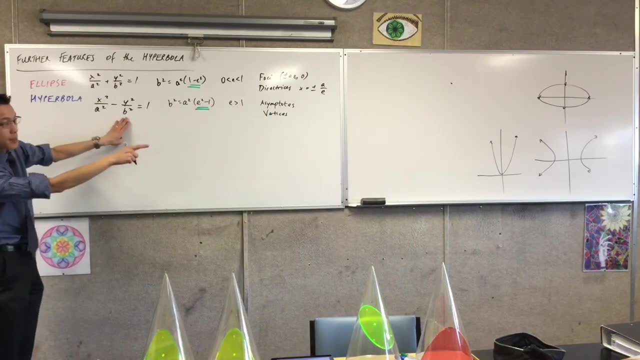 So I don't call these turning points, even though that's kind of what they look like. We're going to call them vertices. okay, Now on this hyperbola, you might remember you can't find any y-intercepts, right. 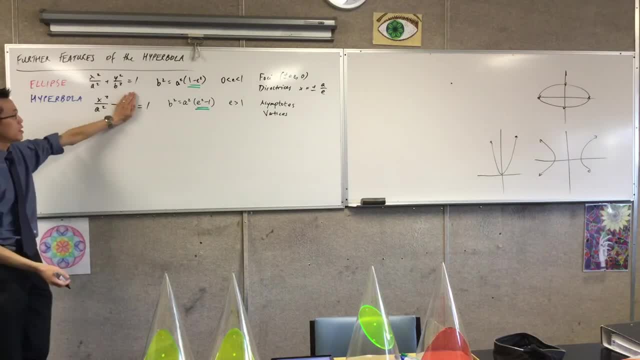 You can't find them, So you look for the x-intercepts by letting y equal 0. So look at that. What are the vertices going to be when you're solving this equation? Plus or minus a right, Oh, a becomes 0.. 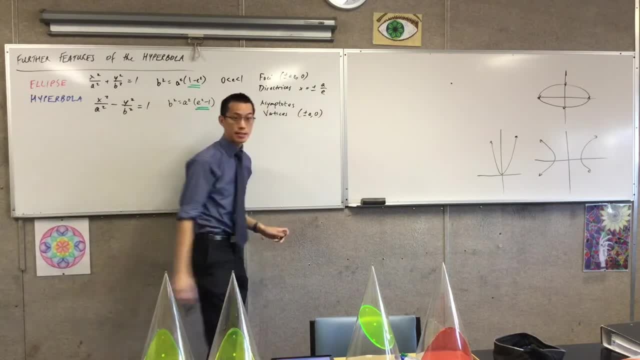 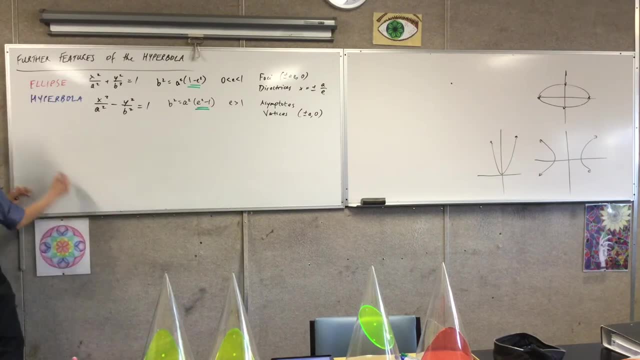 So I'm going to pop that in. That's fairly easy to see. Now let's get to our last piece. Let's now get some algebra back out and let's go off to these asymptotes. I'm going to start by writing the equation in the hyperbola: 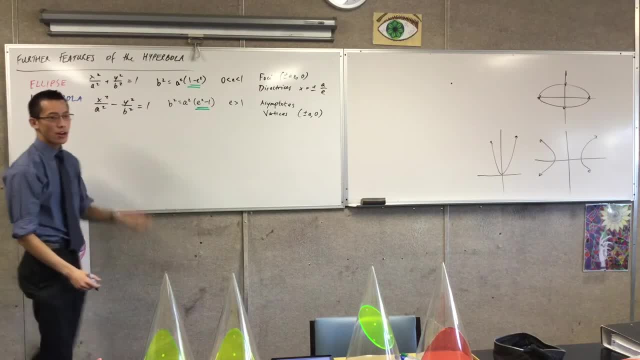 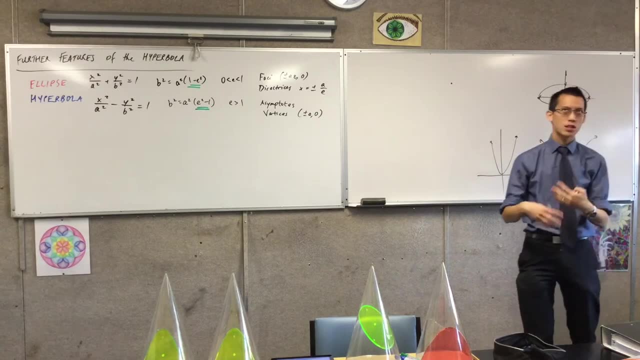 That's going to be my starting point And I want to know: okay, we pulled a bit of a trick with square roots and limiting behavior. last time We saw, I think, for our example it was like the square root of 3 times x. 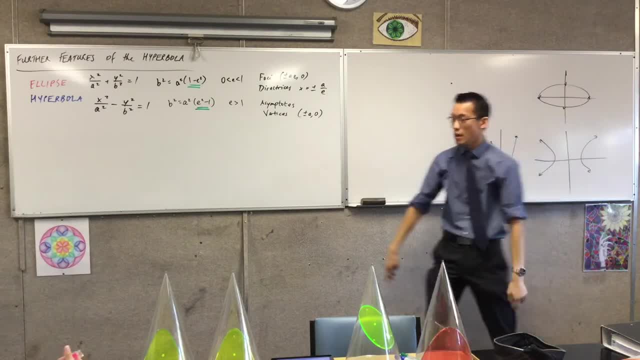 Plus or minus the square root of 3 times x. Those were the two asymptotes we got. So what I want to do now is that same. I want to rehearse that same method, but I'm going to have to deal with the algebra. 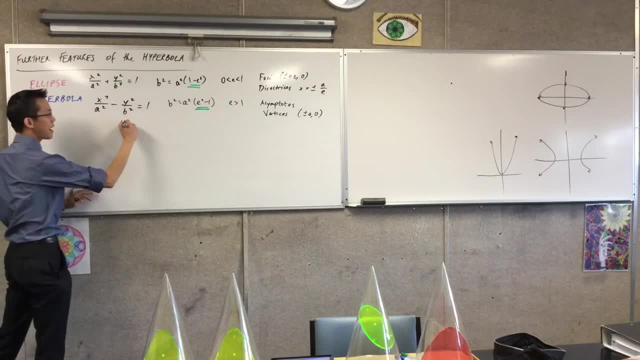 So first thing I'm going to need to get my square and I'll get him on his own right. So it looks to me like if I add him to that side, I'll subtract him from that side. So I'm getting x squared on a squared. 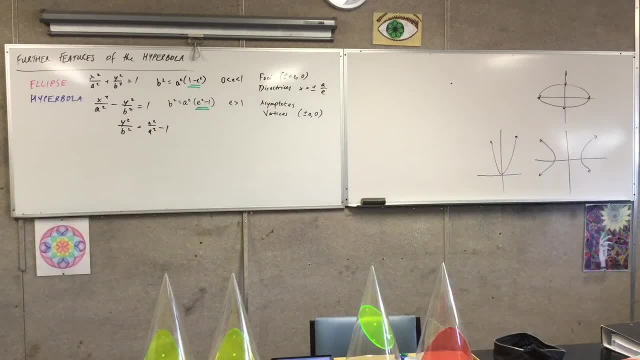 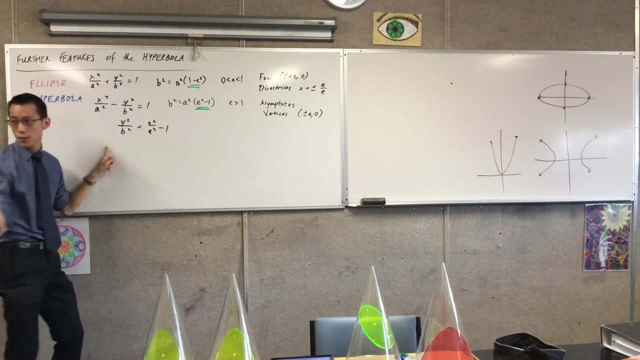 Take one. Okay, this is good. Do you remember what I did after this? Where did I go? Times it by b. Yeah, I'm going to multiply through to get rid of this denominator, but careful, it's b squared. 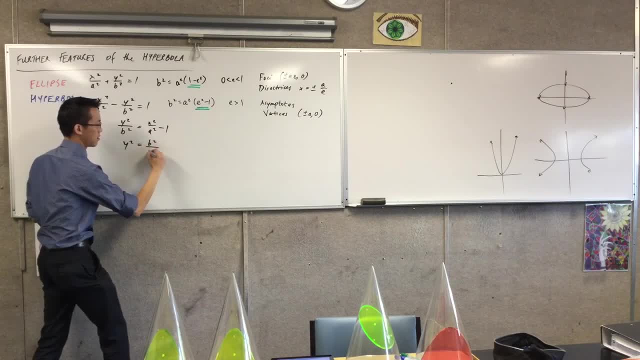 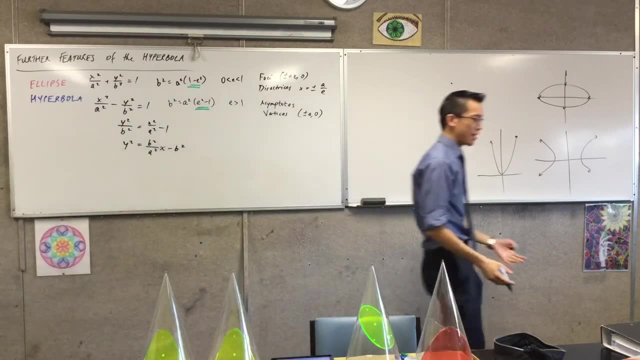 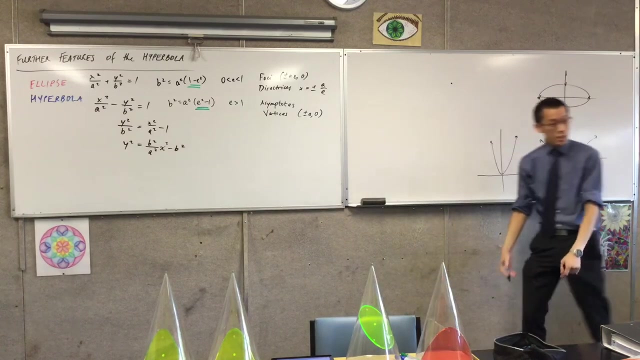 So y squared equals this. Now, at this point, I've got a whole bunch of different things I have to do. Yes, you do. Yep, At this point, I've got a couple of things I could do. I did an awkward factorizing step. 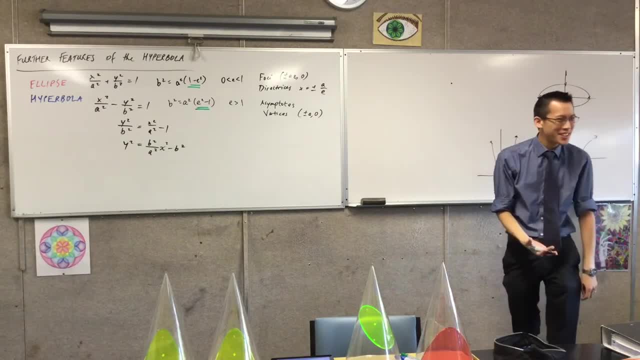 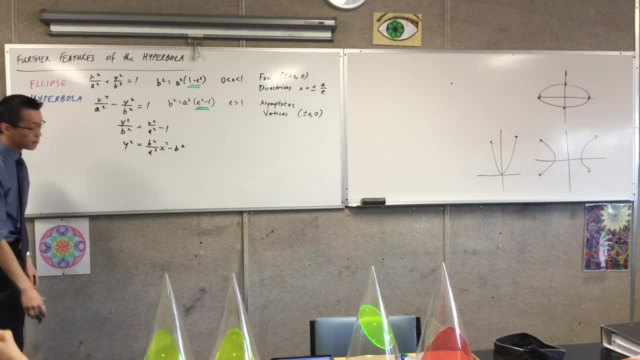 Do you remember A factorization that didn't look very obvious at all, It was very counterintuitive, But it put an x squared on a denominator. Do you remember what I factorized out? x squared? Oh well, x squared. 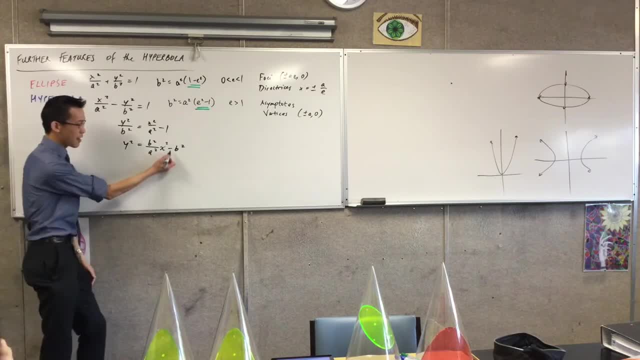 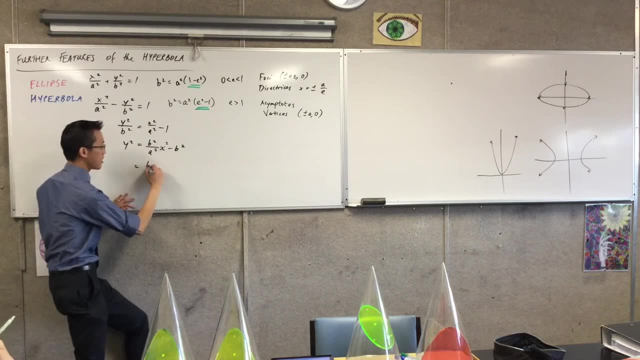 So a couple of different ways I could do it. So basically, I factorized out this whole first term to get one there. Do you remember why the one was so important? It's going to come underneath the square root. So if I bring b squared, a squared, x squared, 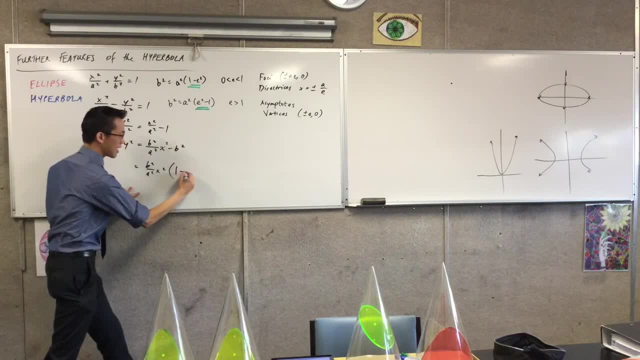 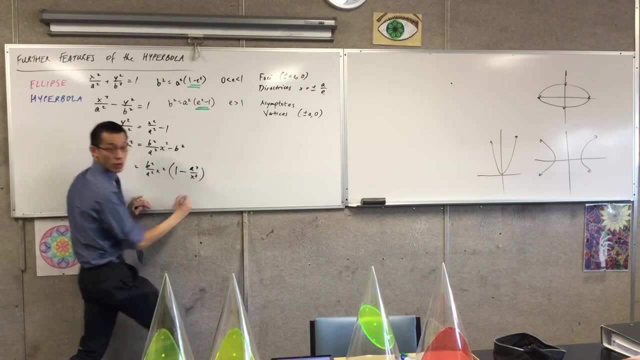 all out the front. you get one. take away Now. just rewatch for a while. There's a b squared there, So it looks like I'm going to be left with a squared on x squared. Does that look all right? And I've got y squared over here. 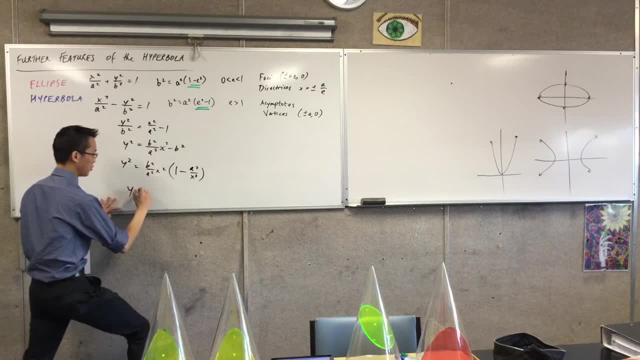 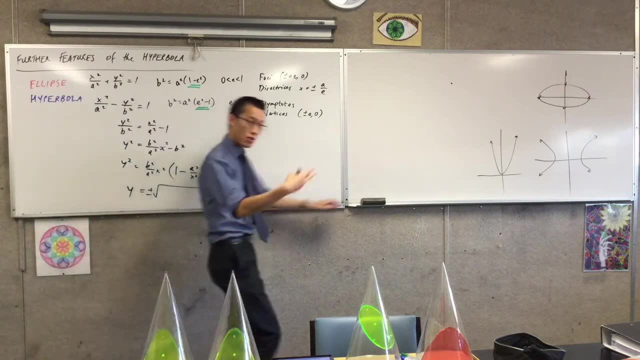 Last step now, before I get to my actual living area. It's plus or minus the square root of all of that. However, I can do this. now that you know what the answer is going to be, You can see all of these things being squared out the front. 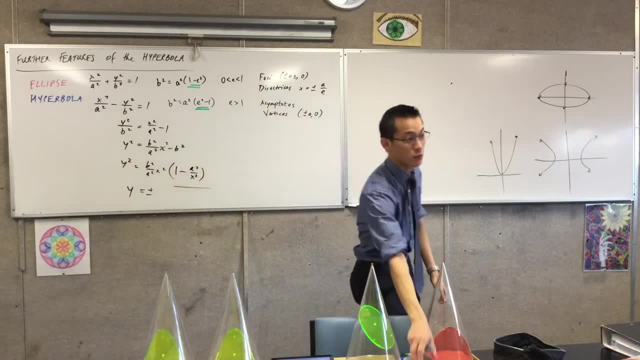 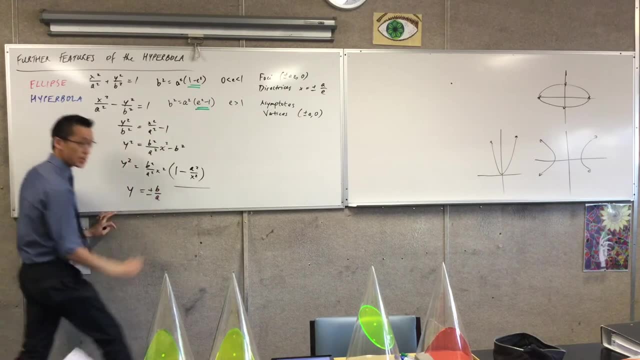 I can probably actually write that right at the beginning and then leave the square root until later. The square root of this is going to be b on a. The square root of this is going to be x. Now, just keep in mind, by the way,